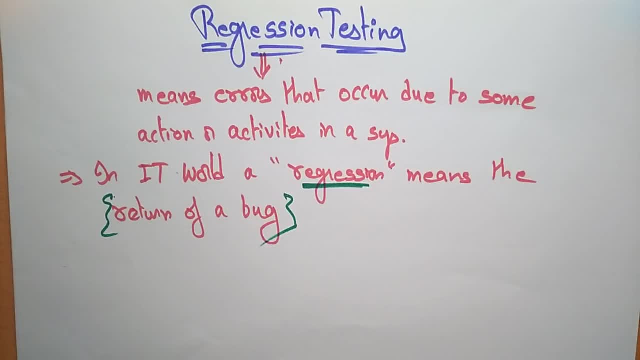 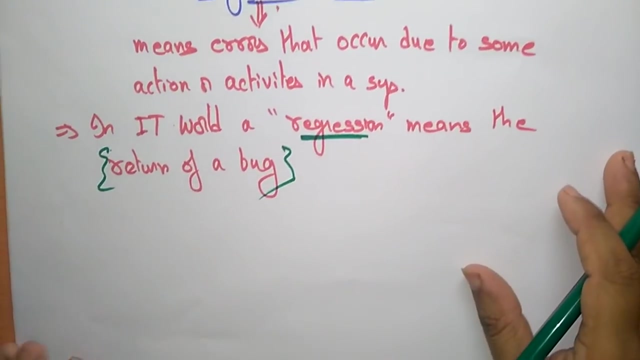 you are rerunning the test cases, the bug is always coming. The rerunning of test cases: if new changes are made, then a bug will be arised So that in that cases you are supposed to do the regression testing. So the regression testing can be used. whenever a new changes are made to your system you have to rerun the test cases again That you call it as a regression testing. Let me write the definition. 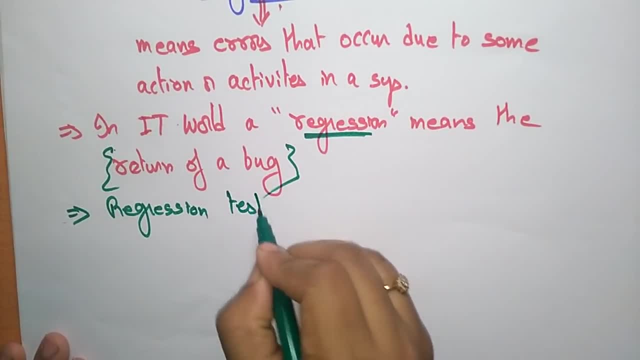 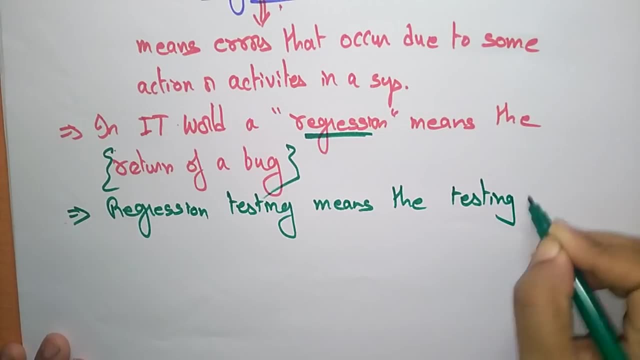 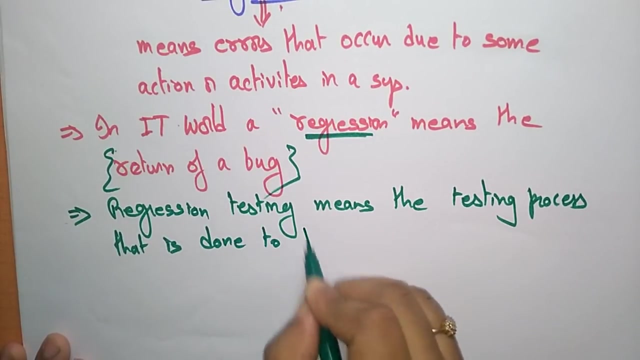 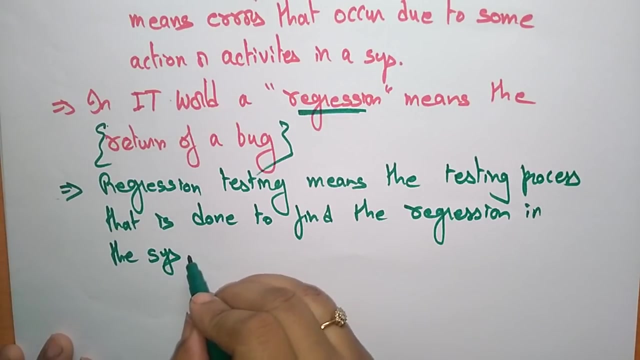 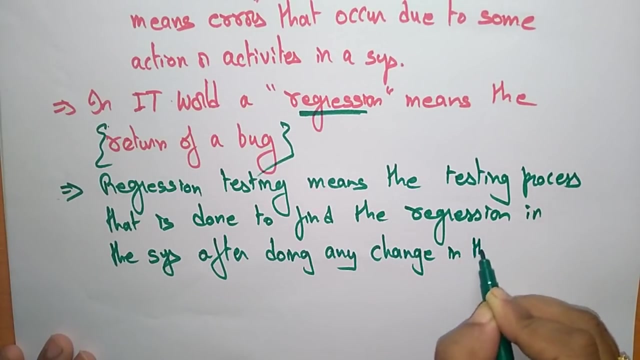 Testing means the testing process. The testing process that is done to find, that is done to find the regression. The regression testing means the testing process that is to find the regression in the system. Now, what is regression testing? It's the workflow app that helped so many people, especially the people who are due to do the test to find the他們. a jogenaofeba ga köna basinci intel bu nnare canvas ke. 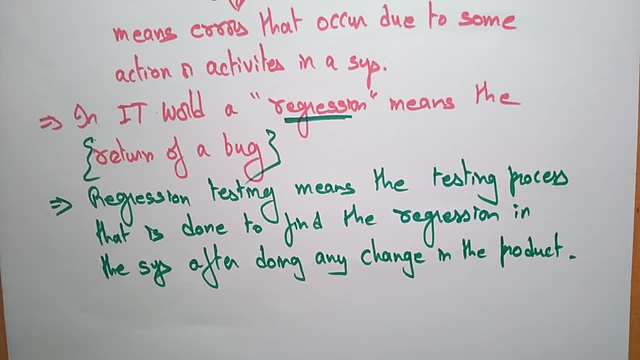 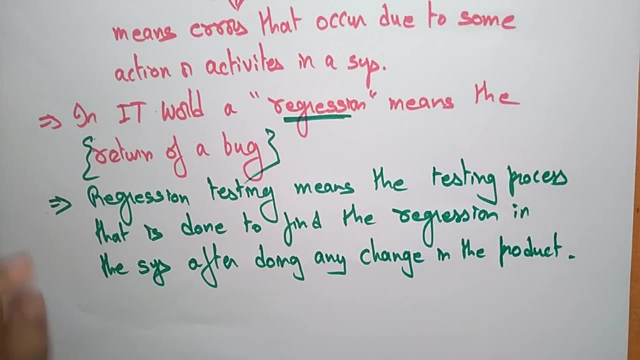 To see the actual change in the product. Well, in this client, Hey, it's something called the risk assessment. So Hey occurs better to follow the regression testing. the regression testing means the testing of a process that is done to find the regression in the system after doing any changes in the product. 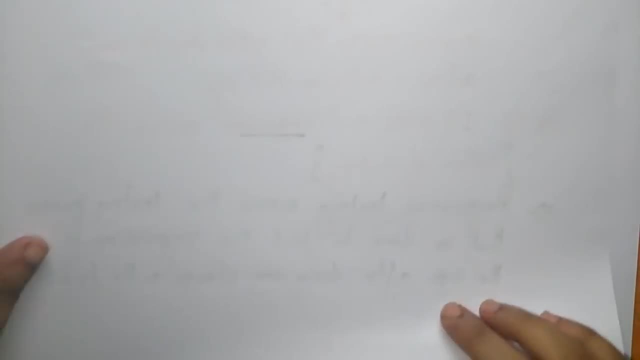 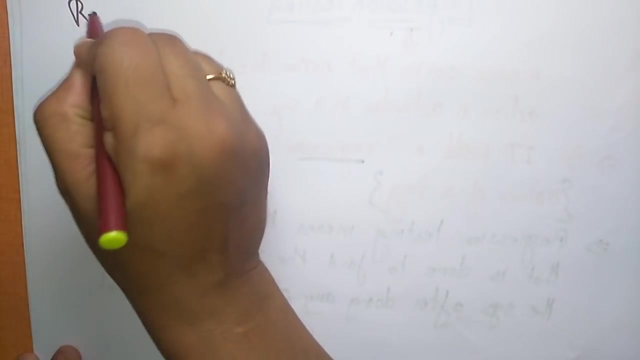 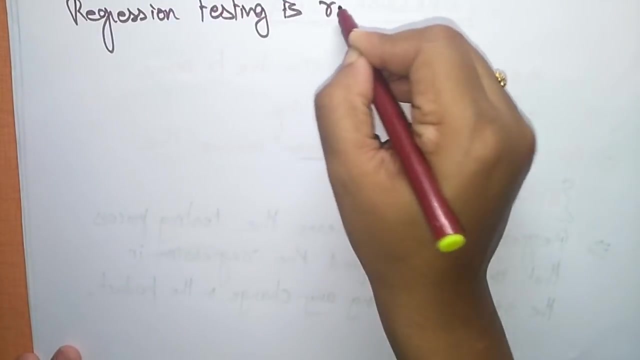 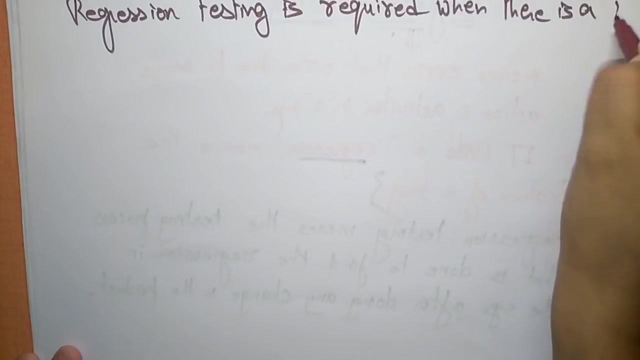 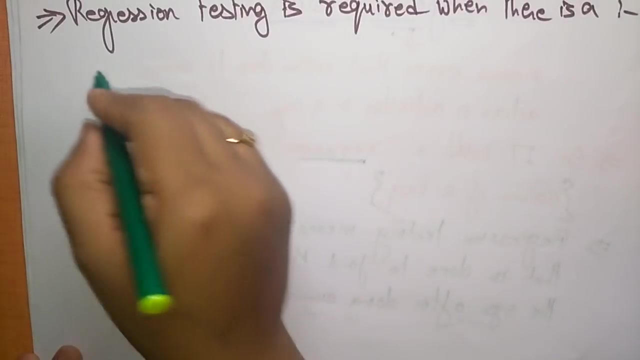 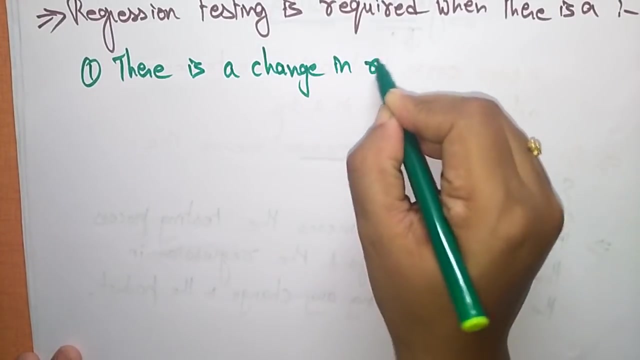 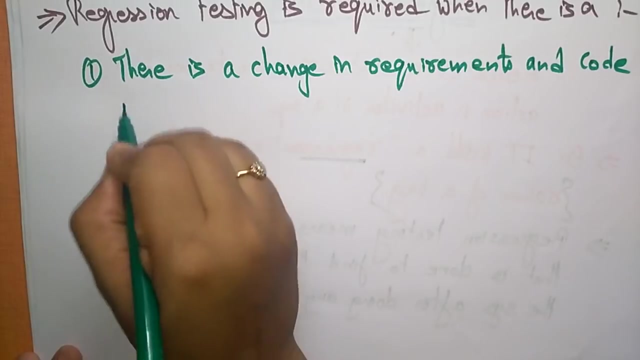 so regression testing is required when there is- let me write those points, that is when it is required exactly. regression testing is required when there is, when there is a change in requirements and when there is a change, change in requirements and code is modified according to the requirements is modified. 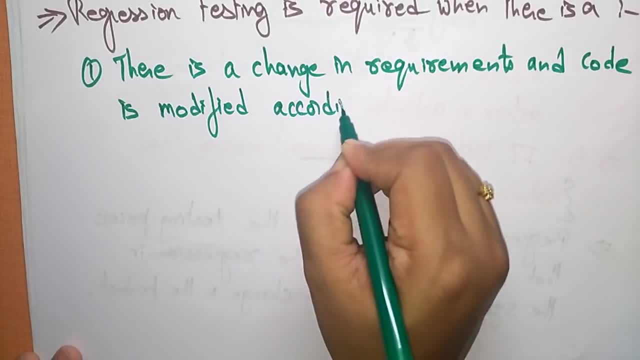 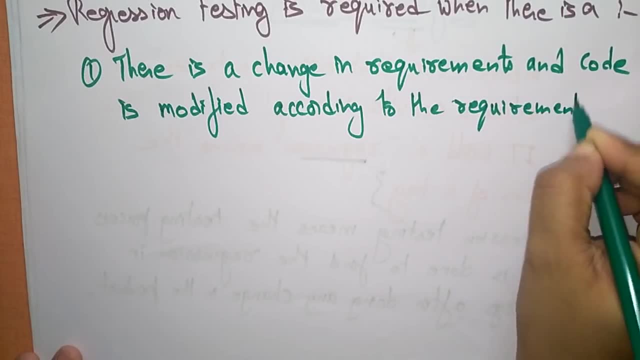 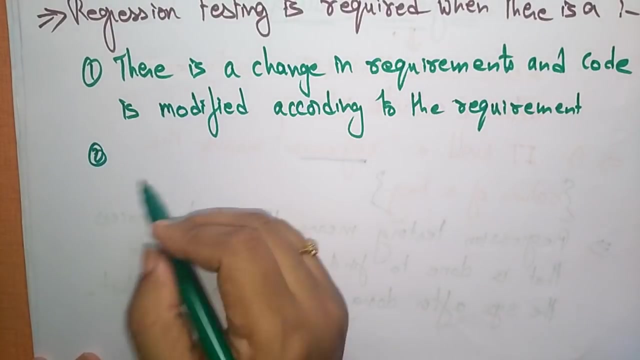 according to the requirements. So whenever there is a change in the system, in that case you are supposed to do the regression testing. So in that case the regression testing is required. So the change in requirements as well as the code is modified. Next, new features. So when the regression testing is required. 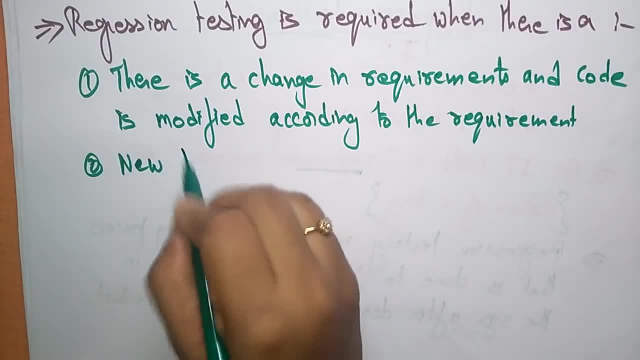 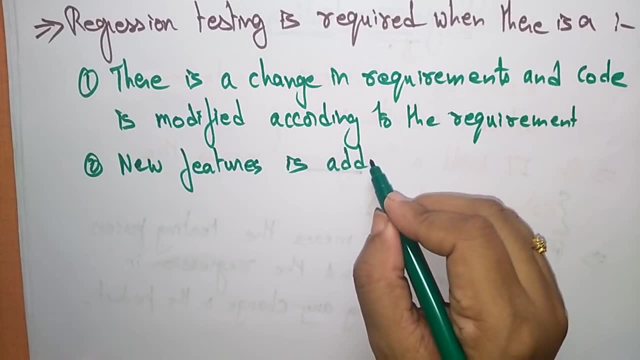 in which case the regression testing is required whenever there is a new feature is added to your system software system. Whenever a new feature is added to software system. So whenever a new feature is added means return of a bug will be raised. So regression testing is required in. 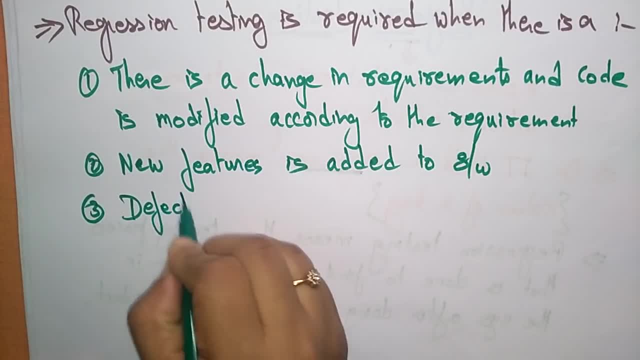 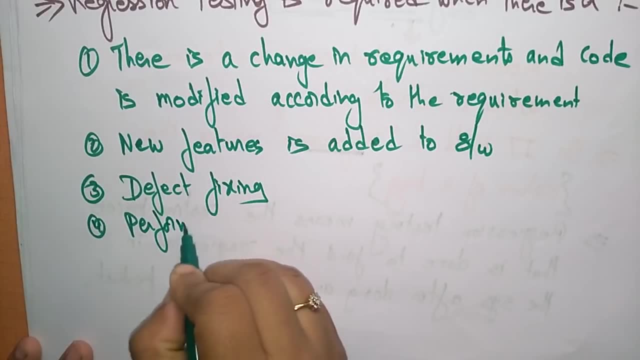 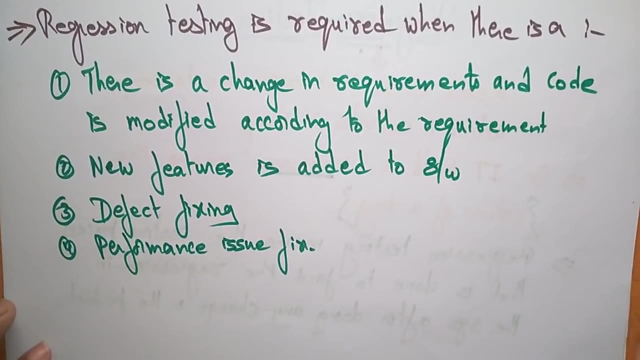 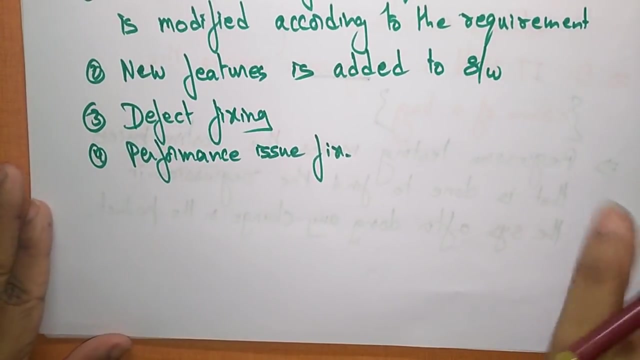 that case. Next, defect fixing. For defect fixing, you need regression testing and performance issue fix, Performance issue fix. So this is about the when the regression testing is required. Now let us see the techniques. What are the techniques that are involved in regression testing? Techniques: 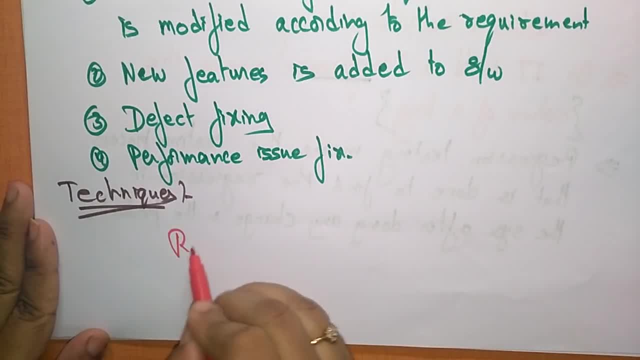 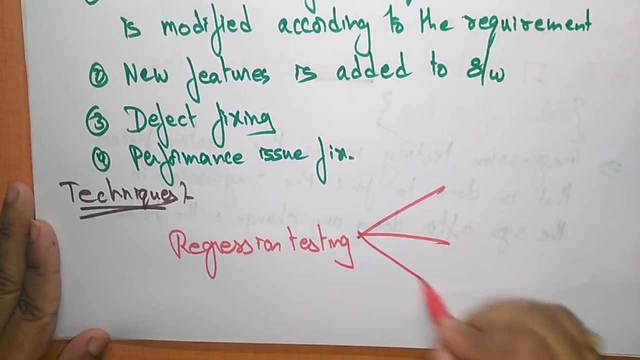 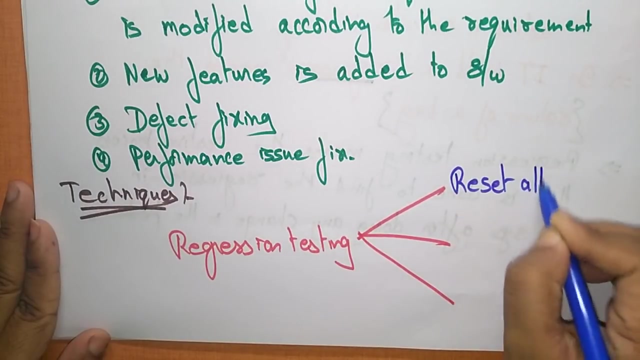 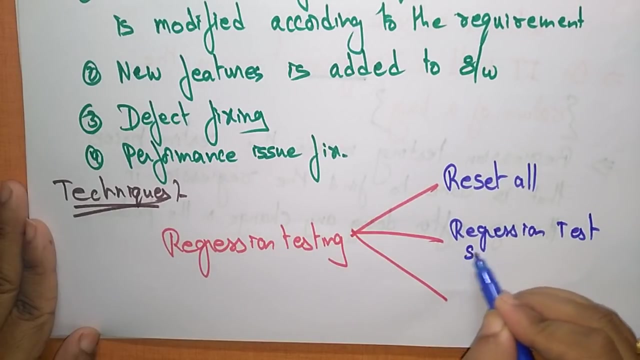 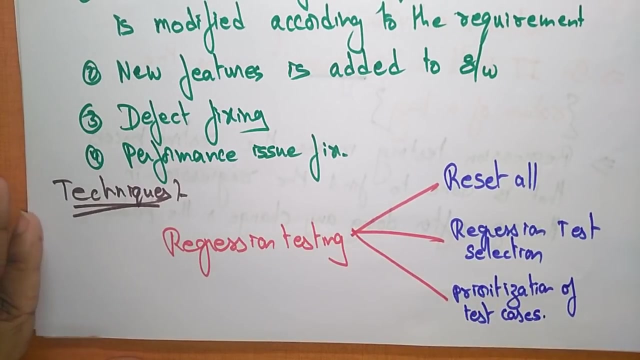 So let me write that A regression testing technique. So there are three techniques are present. So one thing is reset all Another regression, regression, test selection. And the third technique is prioritize- Prioritization of test cases. So these are the three techniques that are there in regression. 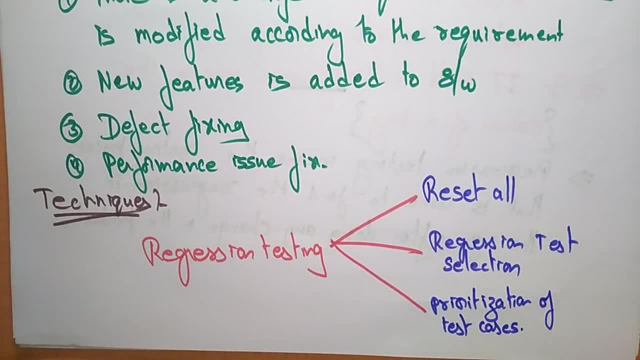 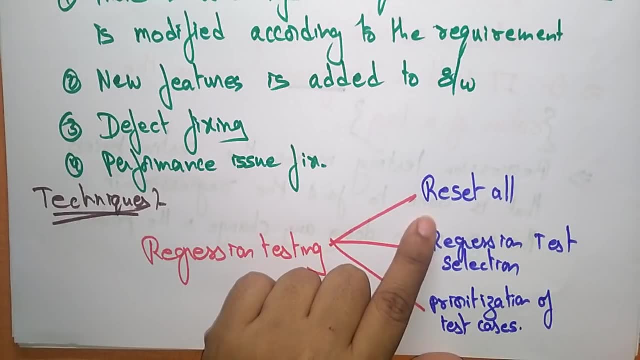 testing. So here reset all means, here all test are re-executed. Whenever there is a reset, all technique will be. it is provided whenever the test are all executed. And this reset all technique is one of the expensive, Because reset all technique is one of the expensive, So reset all. 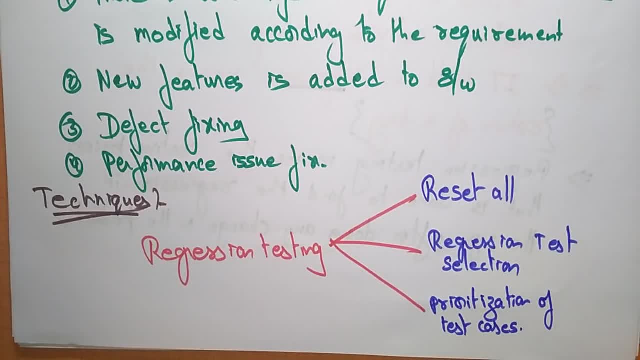 the test cases every time. to reset all the test cases means It is very expensive as well as a huge time resource and resources have to be required. And what about the regression test selection? So when is this technique will be used? So here, instead of re- executing in the reset, all we have F. 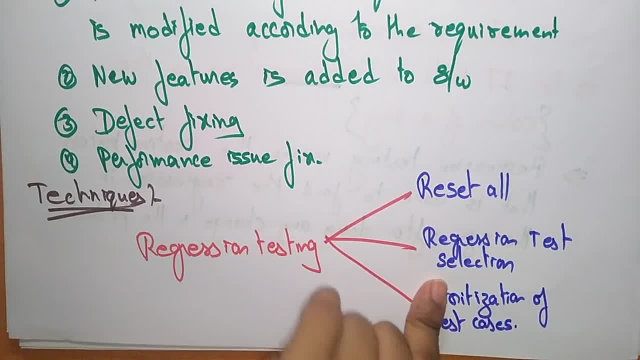 to re-execute all the test cases, But in the regression test selection, instead of re-executing entire test suite, it is better to select part of a test suite to be run only regression test selection means you are just selecting a part of the test case which is having the bug. okay, so.